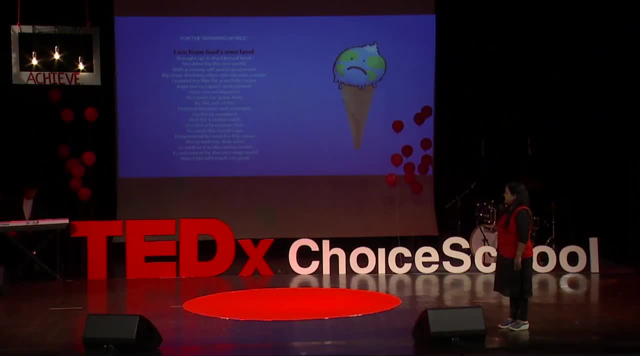 my life I was spending mostly in Annakulam And little while time I was in Delhi and I was say being put me also then little time I was abroad. Of course I tissue my best half and siblings who we are, who are always now. Now they are working here in Middle East as well as in. 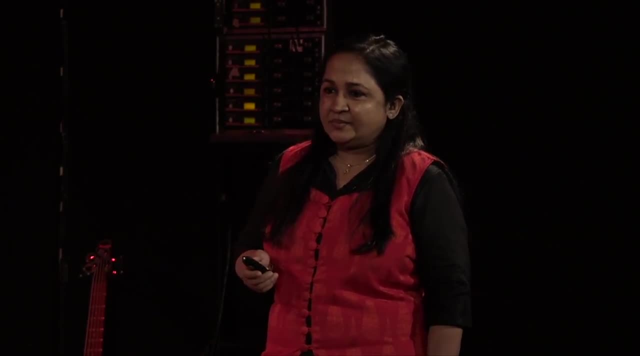 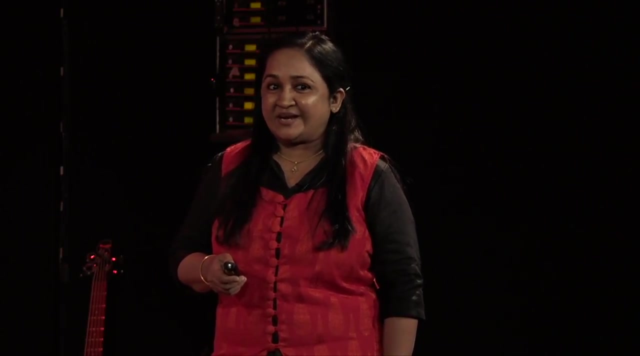 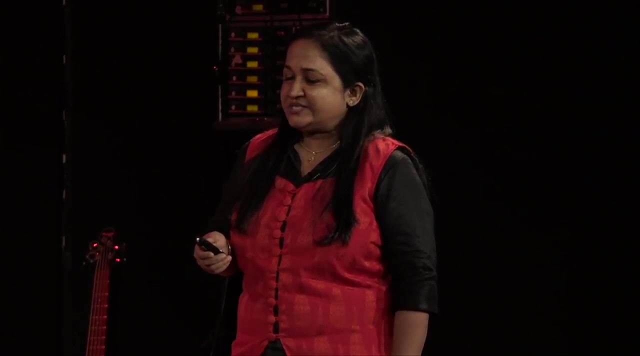 america and also the places, because now i'm working as senior town planner, i am working here alone and all my family members are away. that you must understand. that's with a dedication to practice my theories. i'm, that is, i'm remaining here and i'm working here as senior town planner. 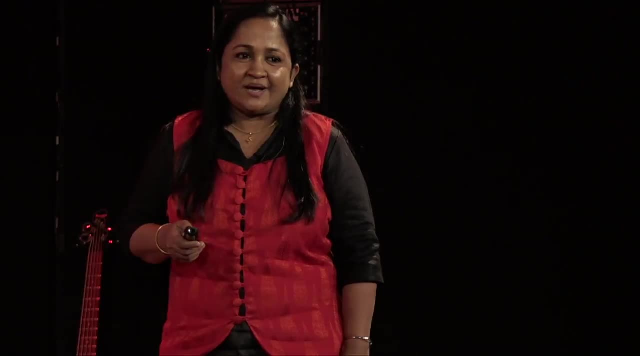 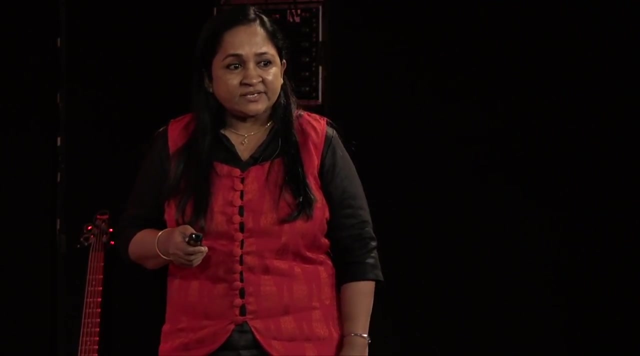 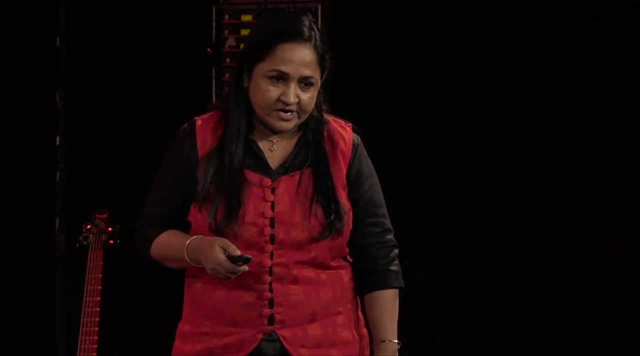 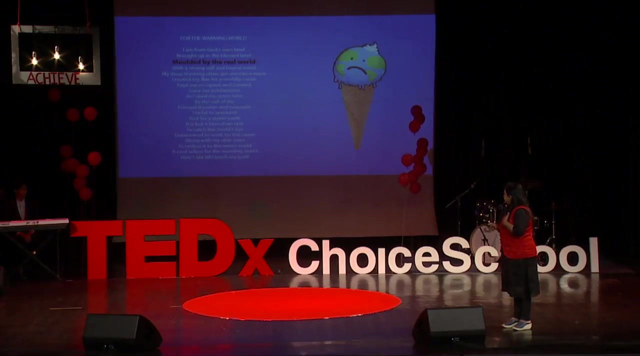 now in greater coaching development authority- i'm the head of the department there- and on the on the expectation that i'll be getting getting some chance to practice my theories, which will be beneficial for my city and in turn, it will be beneficial for the entire world and my characteristics. i myself, that is, i myself decided and i know myself, that is. i have got a. 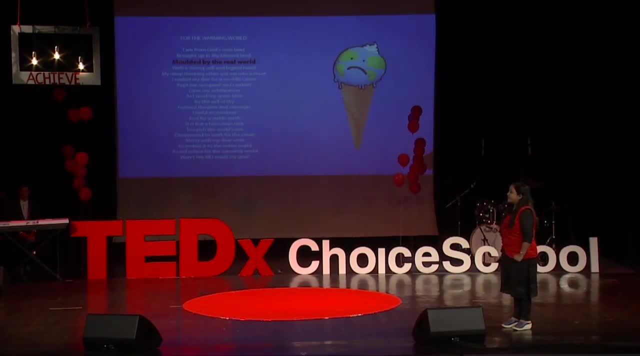 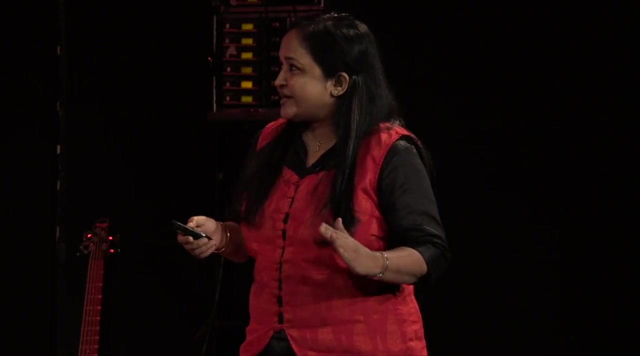 strong will and also have my strength. this i have got a logical mind and i, of course, maybe positive or negative. i had the habit of deep thinking which i started thinking ago about myself. i found that it is not the, it is not a right thing to do, because life is to live, not to. 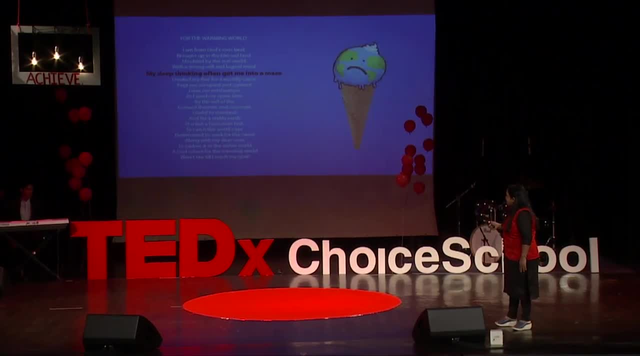 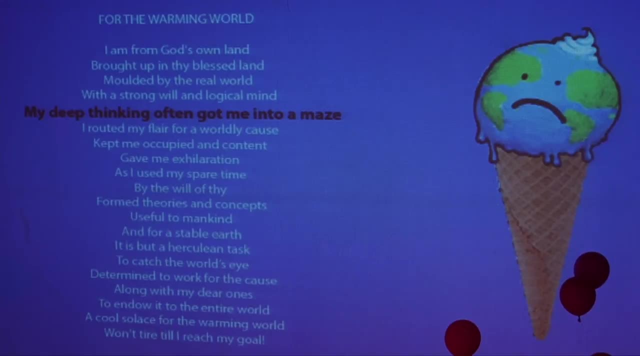 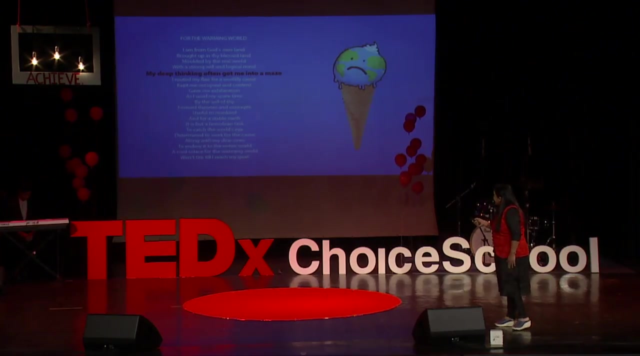 think much. so i rooted my flair because i always wanted to see that all the negative things, everything has got a positive. so i just wanted to fit my characteristics, my ability, to a positive thing, so that and that i wanted. i rooted my flair for a worldly cause that is kept me occupied and content gave me acceleration. 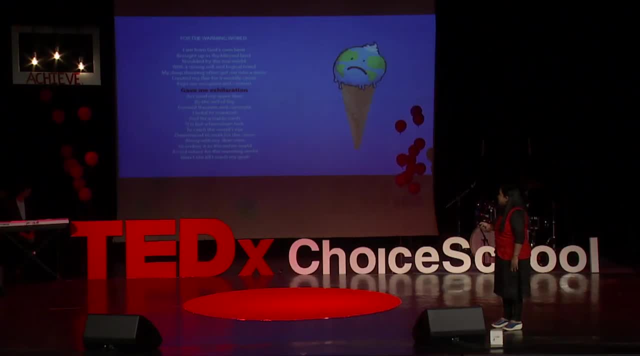 as i use my spare time, because i never compromised my job, i never compromised my family, the spare time i have used for for the betterment of the world and i rooted my flair for the vertic cause of global warming, but the will of die, because i 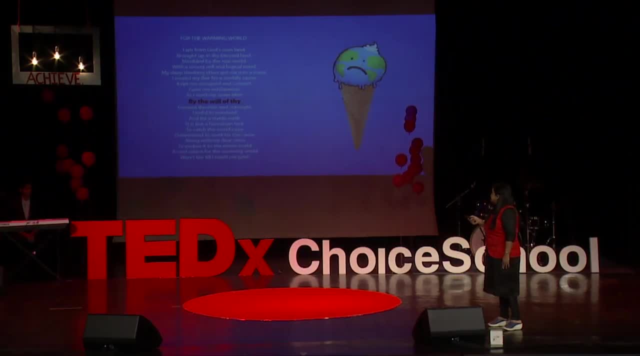 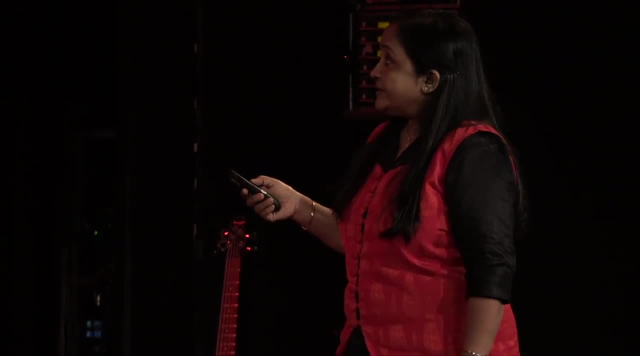 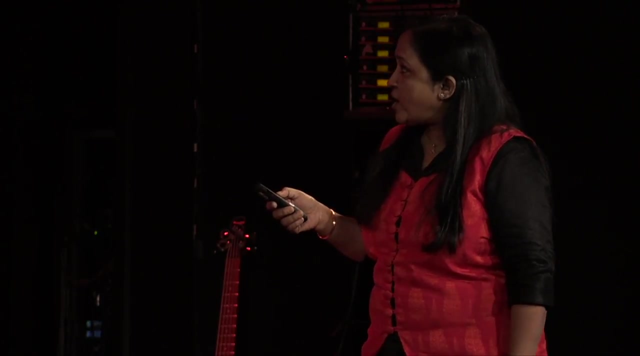 always believe in god. i am a strong believer of god for theories and concepts useful to mankind and for the stable earth. but for but it is but a herculean task to catch the world's eye, determined to work for the cause along with my dear ones, to endure it to the entire. 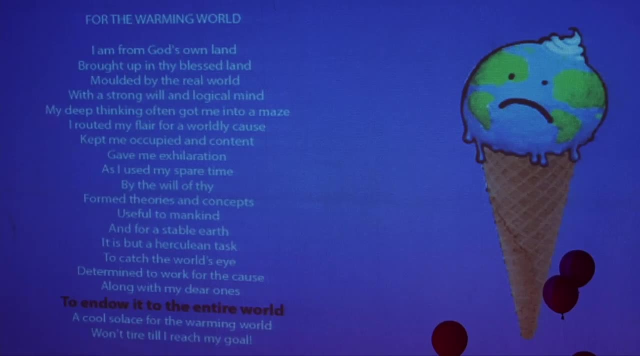 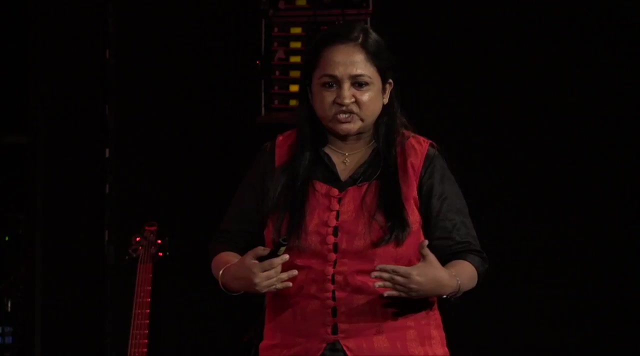 world, a cool solace for the warming world one time till i reach my goal. that's the point i i hope you all first you might might have got some idea how, because everything my flair it has come internally, not for externally. i myself had to sar discounts. are we really happy and condom? or thats why i are ordered? 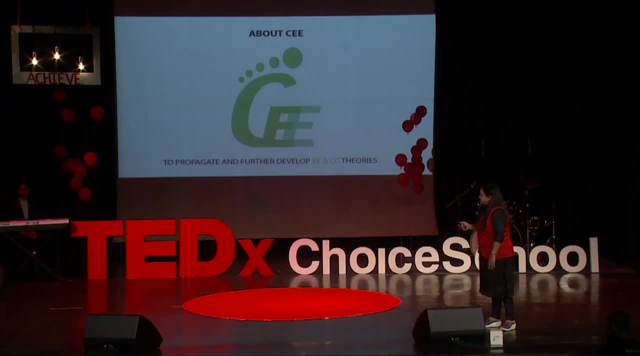 applaud myads, butst broadcasts, I think, thoughts entitled. and there they are going to find the second day of my blankets, but they don't quite dot Maxwell. but this that i mean gee, you mean my name. send a phone: anderman the fifty Hanseatic, to propagate and further develop the EE and CC theories. 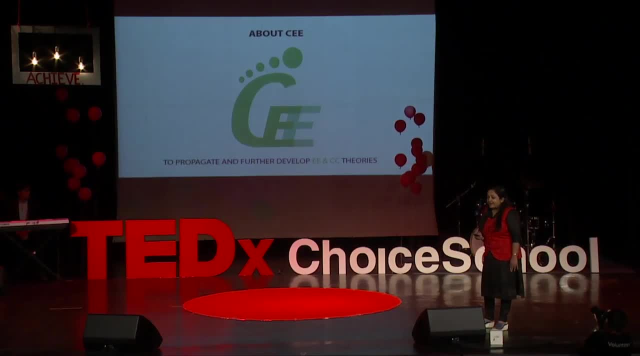 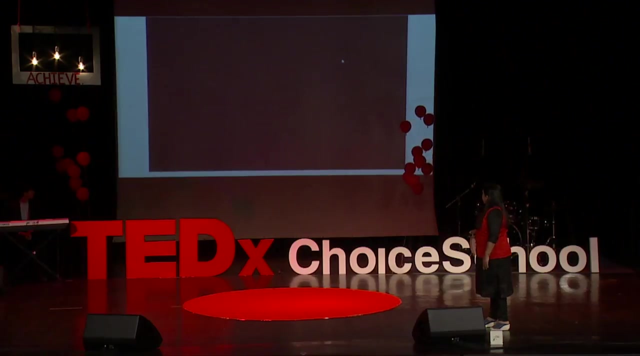 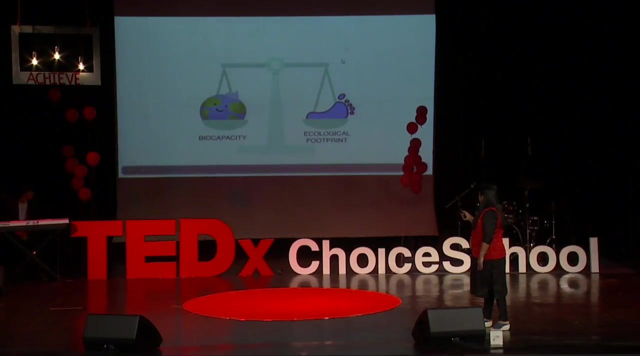 which were evolved by me during my PhD research in 2011 from the Cochin University of Science and Technology- Cochin. Yeah, EE and CC theory. I always. I already told you that is through my PhD research and for which my CE has been formulated. 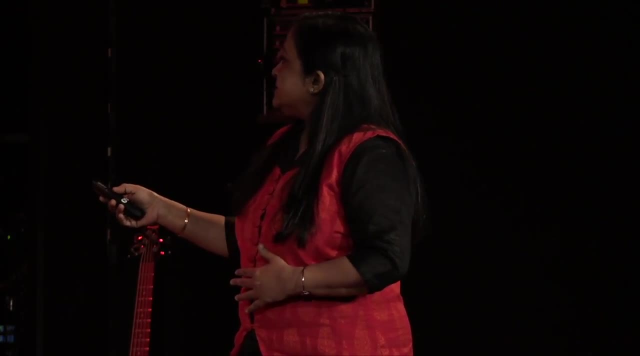 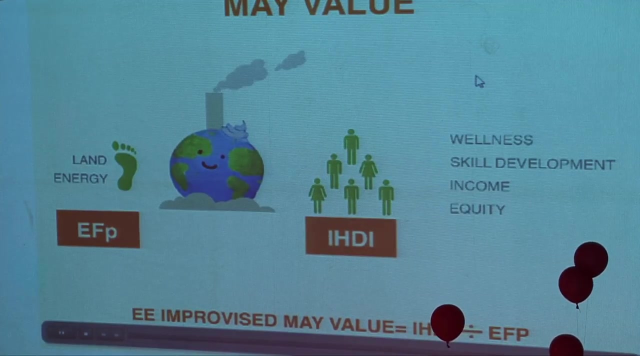 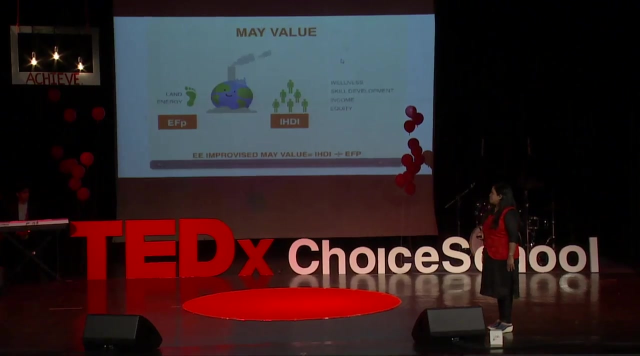 And further. I have improvised my CE, EE, Environmental Efficiency to May value and I improvised my carrying capacity to tone value. And I will explain what is May value. Because Just imagine Earth is a factory or it is a machine, So something is produced there. 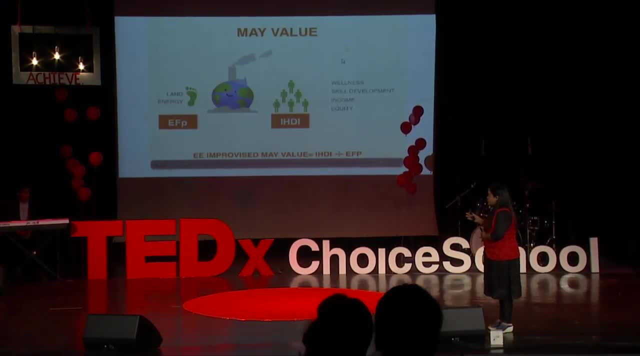 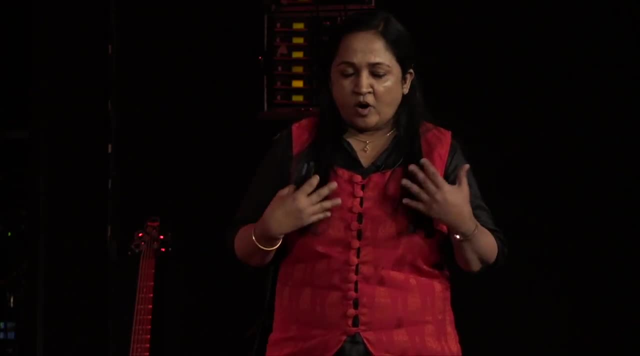 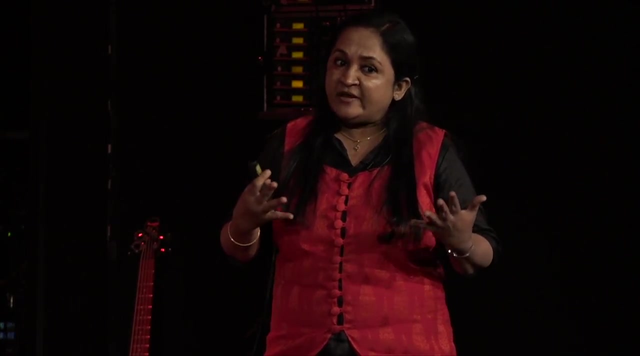 It has got an inlet input as well as an output. What is input? That is ecological footprint. That is all of us will be knowing. what is carbon footprint. Ecological footprint is the terminology invented and propagated by World Footprint Network. 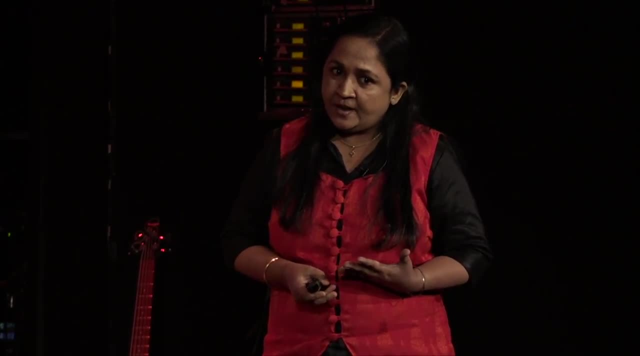 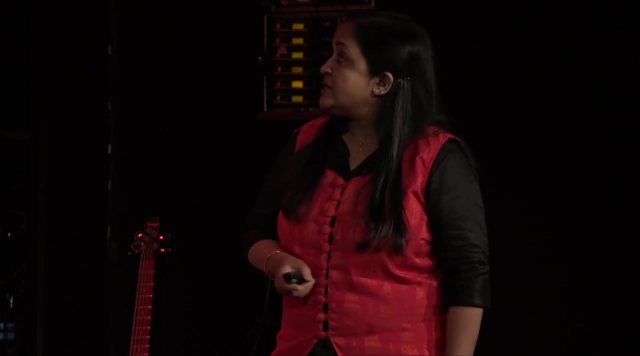 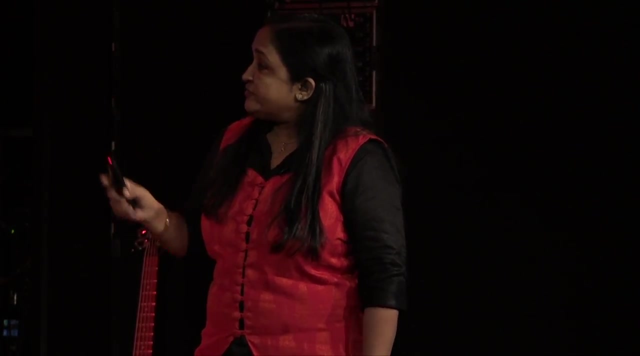 which is headed By Dr Mathis Wekernagel And it has been propagated by WWF. I got the idea of an ecological footprint concept from Dr Mathis Wekernagel And this input, input I have taken for the machine like Earth. 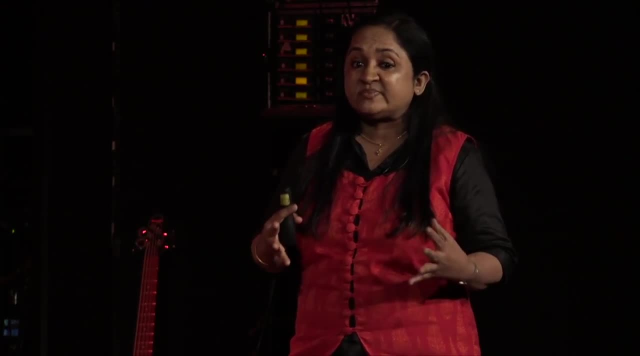 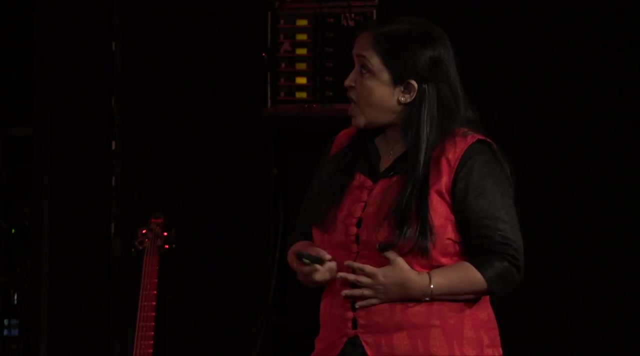 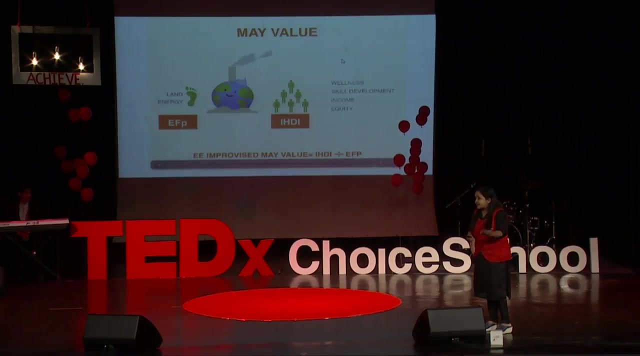 input is the ecological footprint. That is the per capita consumption of an individual, average Indian average man. That is ecological footprint. In short, if I say, telling that it is that sum total of land and energy, energy it is again converted to land, land. 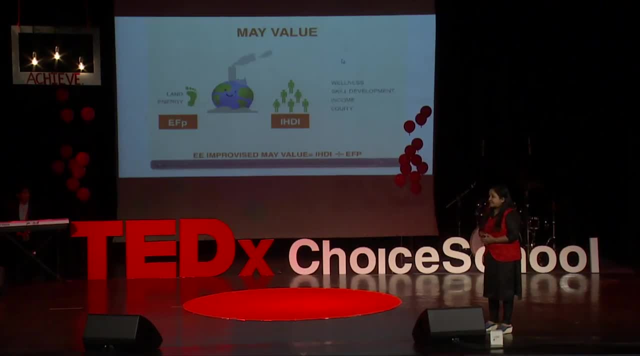 what we are using. energy is again converted to land. the amount of land required for sequestrating the carbon dioxide, so that everything is expressed, ecological footprint, is expressed in global hectares. and what is the output? it is- again, i will say that i have taken the idea of that is. 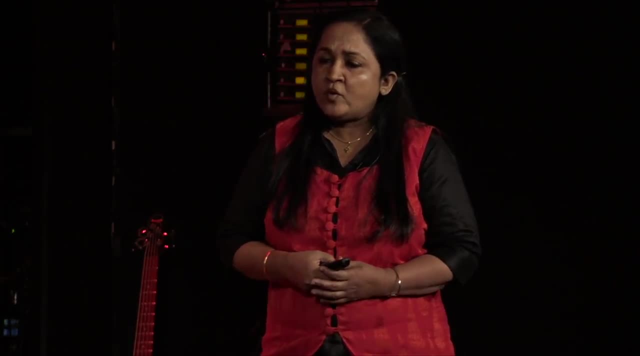 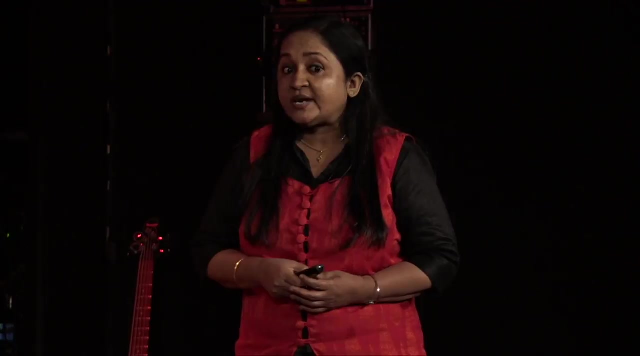 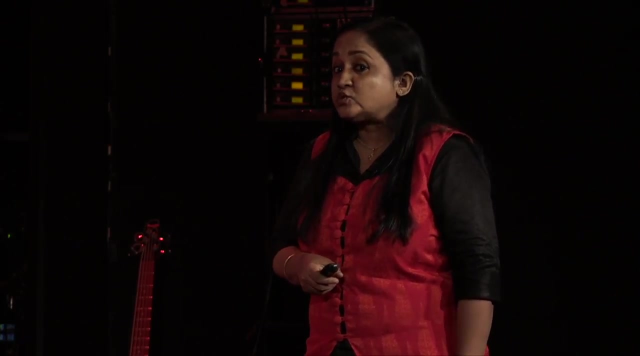 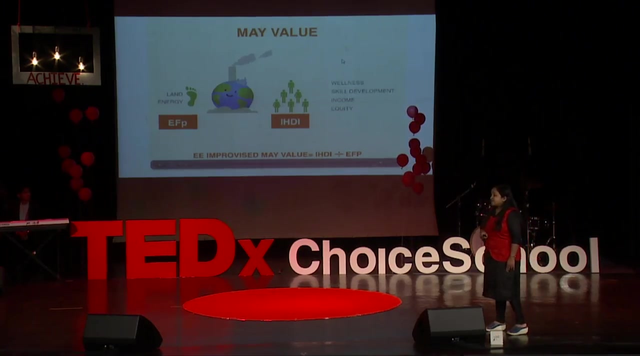 undp, united nations development program- they have formulated two things. one is human development index, which is characterized by health, education and income. and in my language, health, i have modified to wellness, education, i have modified to skill development, and again income, income the same thing. and then, in the case of ihd, in inequality adjusted human development index. 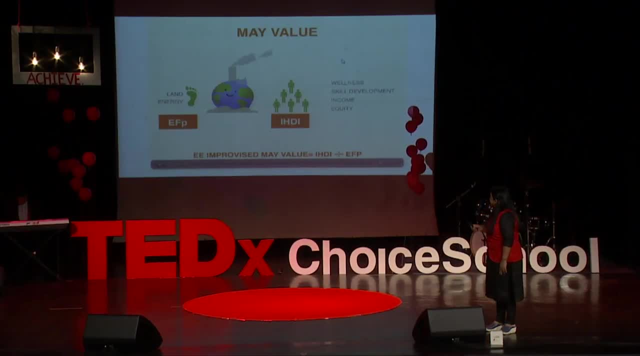 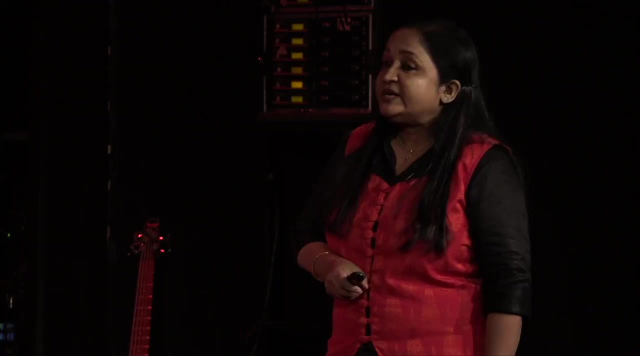 formulated by you and the dp. from 2010 onwards. they are considering the value of equity. also, inequality adjusted human development index. they have formulated- and i have made this ee or may value as inequality adjusted human development divided by ecological footprint. that means we are getting in, quantified, we are 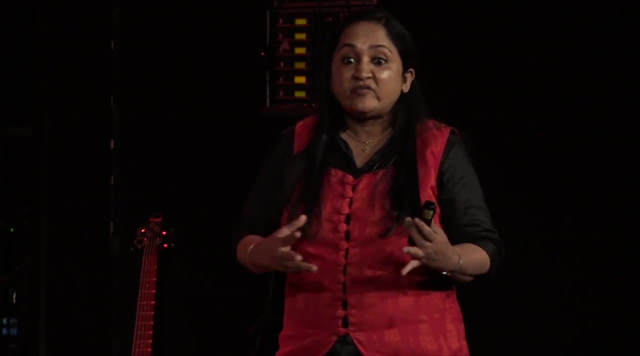 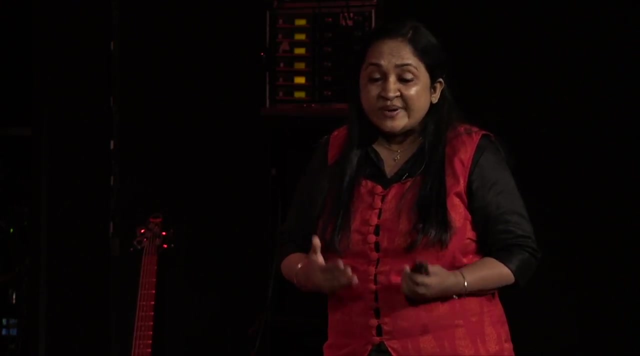 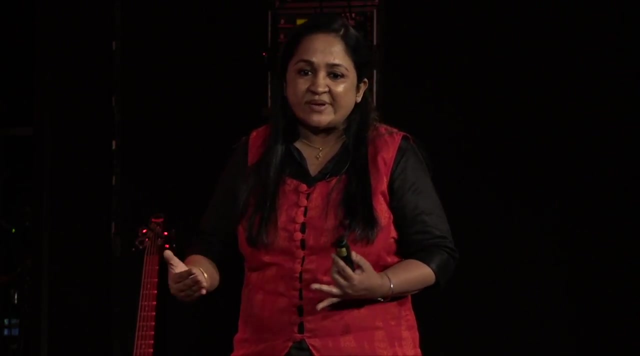 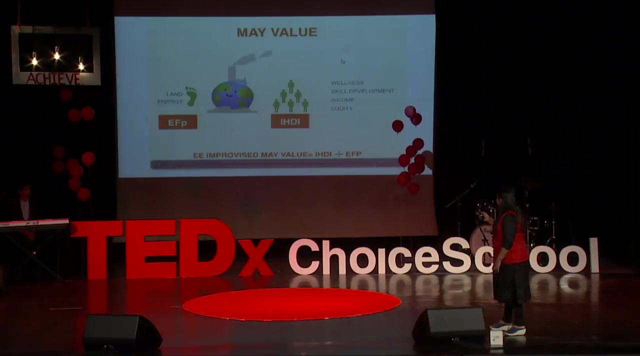 getting in terms of numbers? what is the environmental efficiency of the world, environmental efficiency of this country, that country, so that now human development wise, very high values of countries may go down? what is their human development achievements with respect to inequality? adjusted human development, that is, may value. 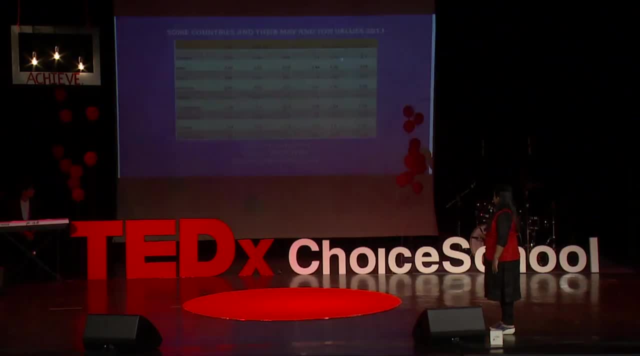 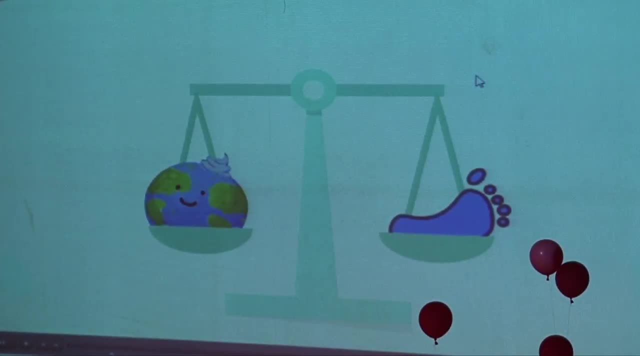 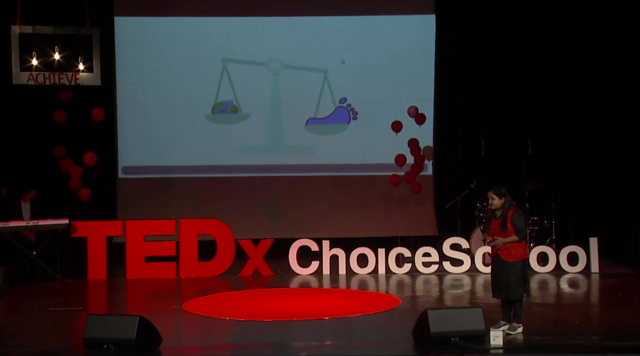 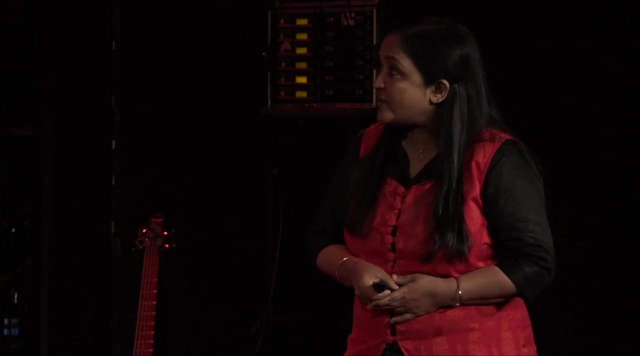 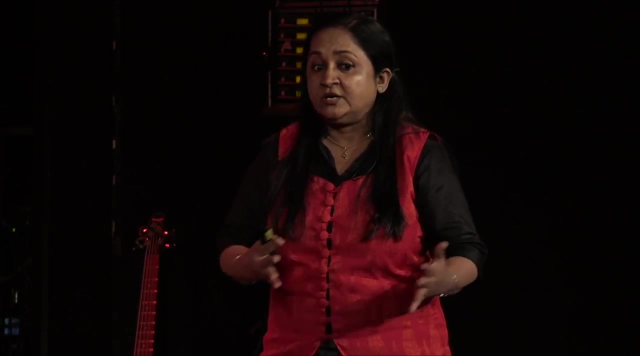 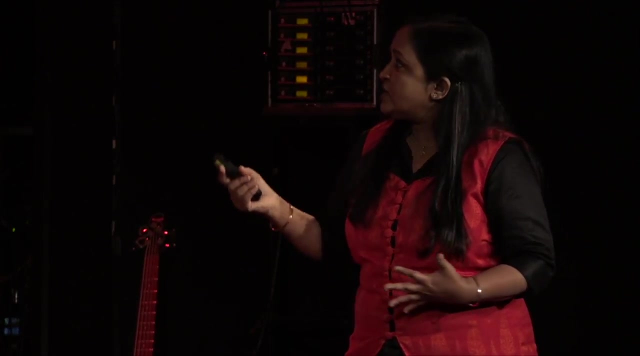 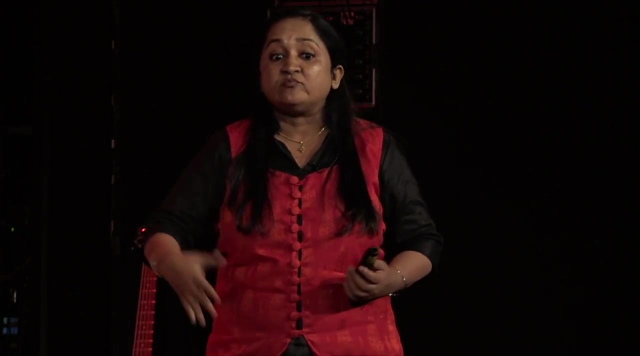 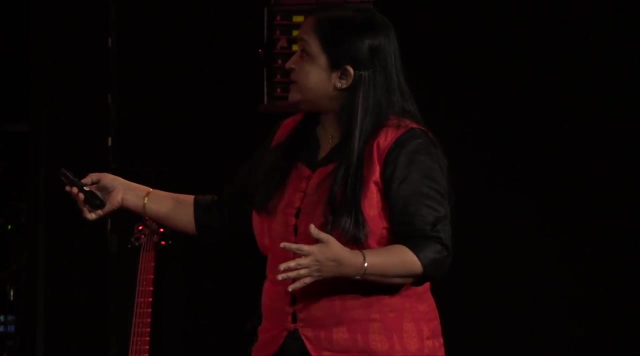 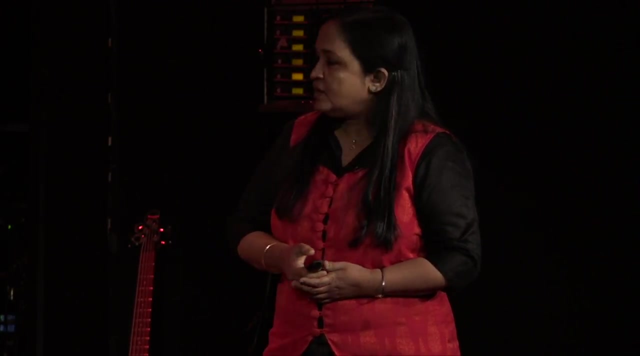 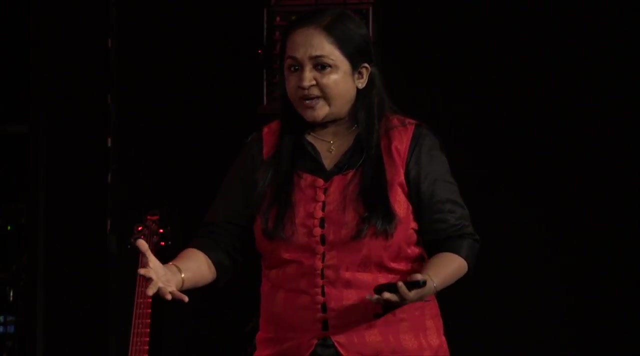 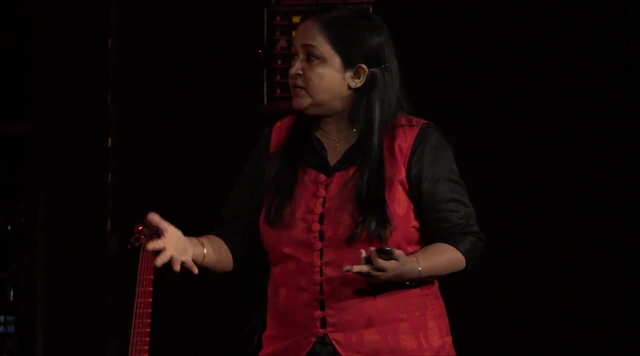 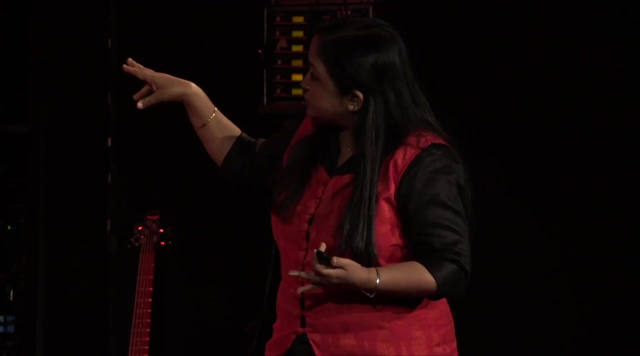 so would be the world world. so what is the? what is the comparison between what, what we have, that is, biocapacity, and what we are consuming? and if you are, if you are consuming more ecological footprint, ton value is negative If it is with respect to bio capacity. if you are consuming less ecological footprint. 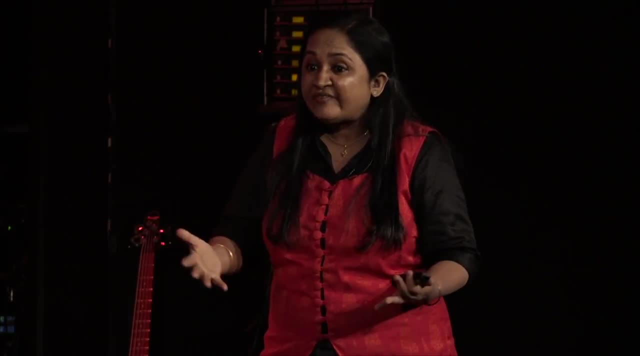 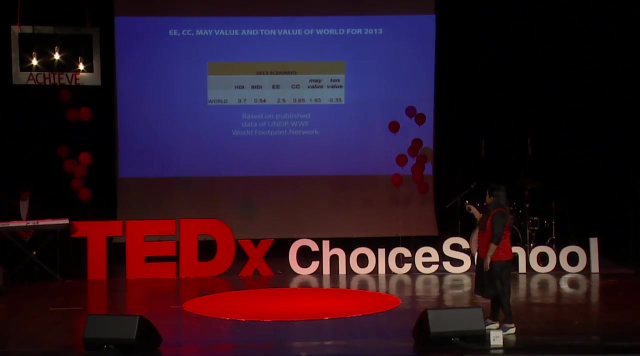 that means ton value is positive and if it is balanced, ton value is 0.. So, based on the that is database from UNDP and WWF, I have calculated this: HDI, IHDI. these are all the figures we have taken from the WWF. that is UNDP site, but EE and CC. 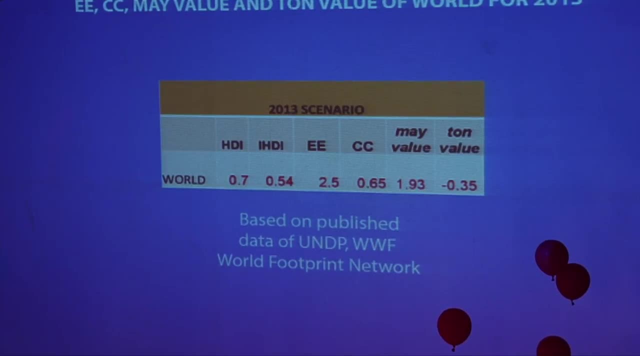 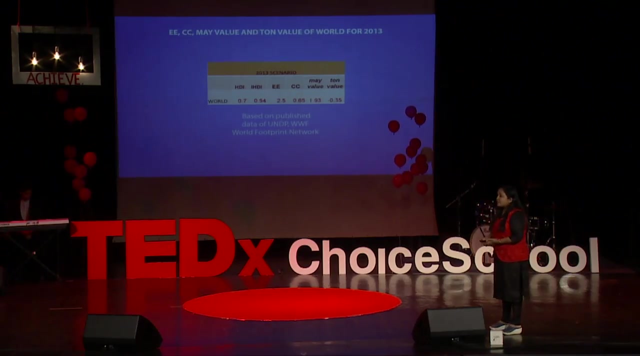 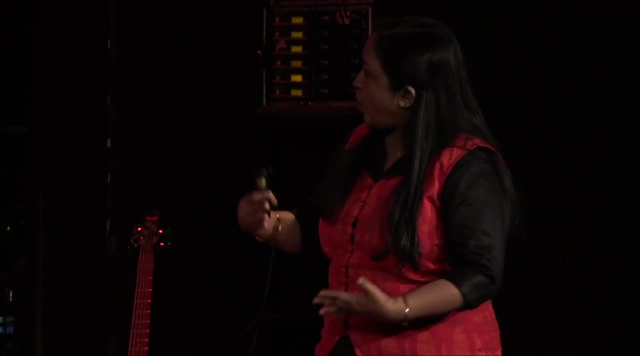 value I have derived it is 2.5 and 0.65, but may value is that is IHD by EFP. it has again come down because so much of inequality is there. So this HDI is existing in this world, which is quantified. that is may value. it is going. 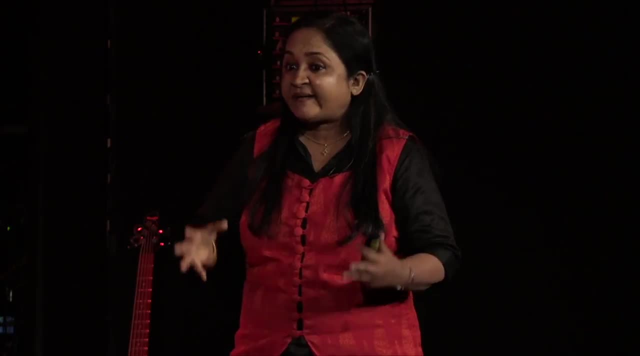 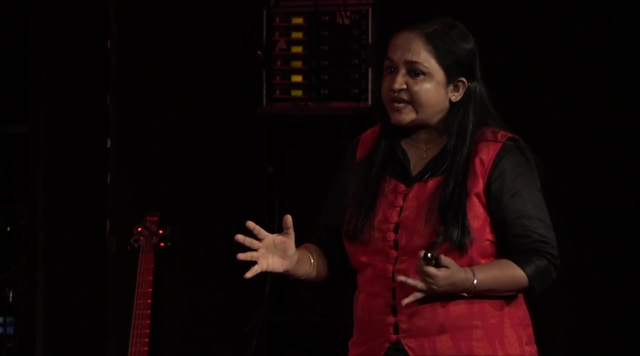 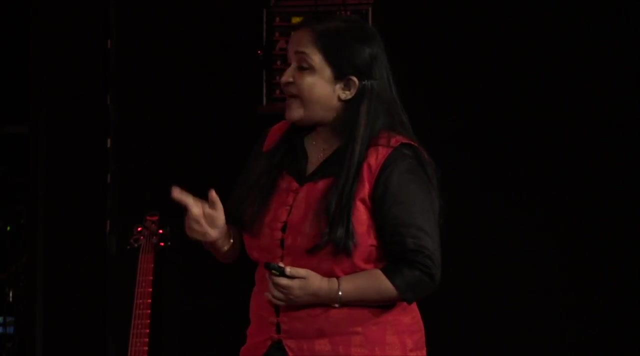 down. that is inequity. adjusted may value is the crux of everything about our achievement and ton value is negative. that means ecological overshoot is taking place. we are consuming what more than what we have. that is the indication, and at least ton value should be. 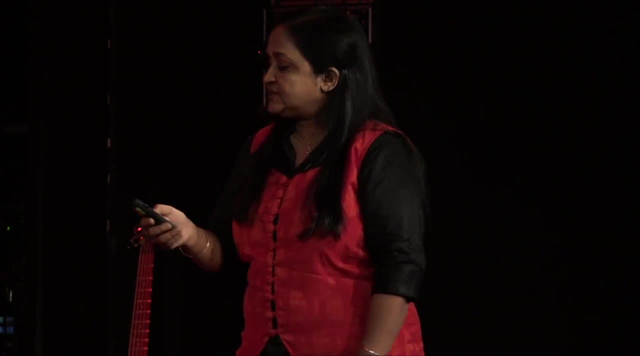 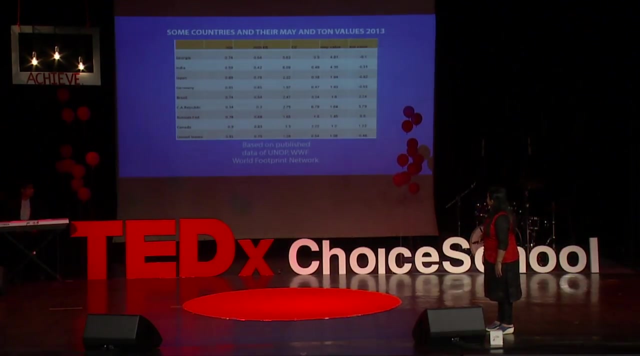 0 and should be non-negative value. that is the favorable condition And these are for that In the countries, some calculations and see that in the Canada, in the case of Canada, may value is 1.2, while this EE is 1.3, that means little bit of small gap is there with. 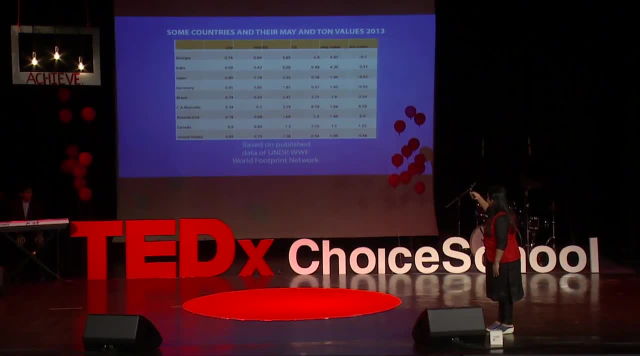 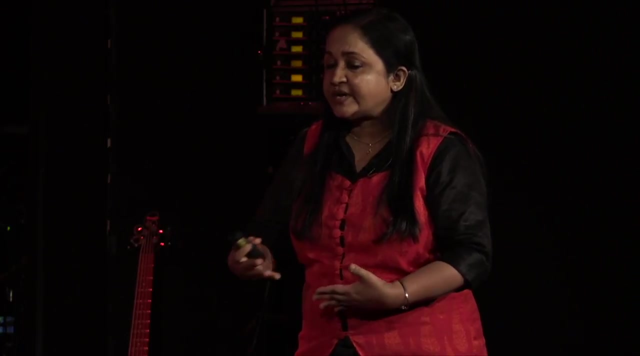 respect to inequality. but in the case of countries like that is India, this EE environmental left shift 6.09, while may value has reduced to 4.35, that means inequality gap gap between the US and Canada. that is crap. it is a half and half, not its. it is more. that is the 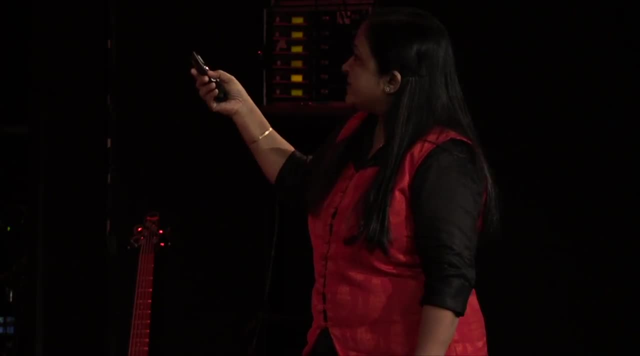 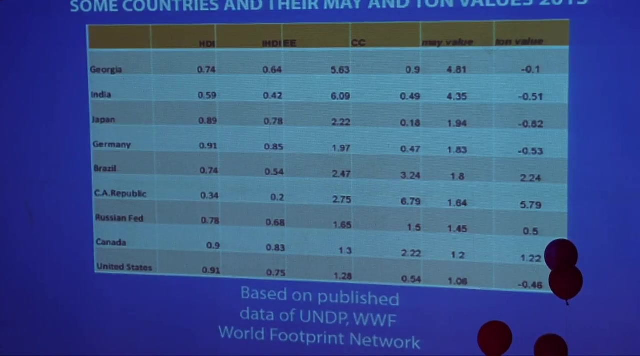 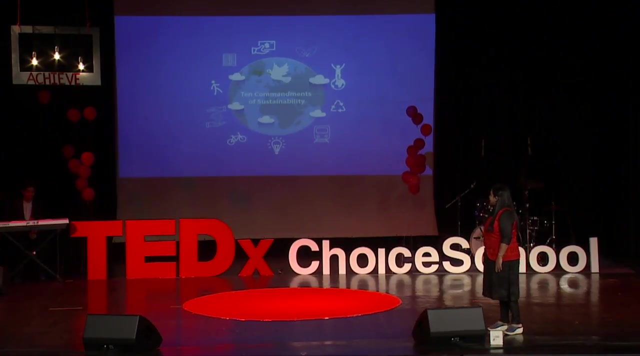 indication And the case of ton value in some of the countries. see that in the Canada. it is positive. that means they are having much resources with respect to their ecological footprint. Based on this, I have made 10 commandments of sustainability. 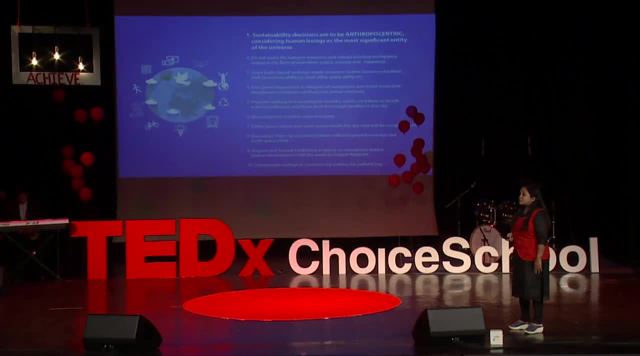 Sustainability decisions have to be anthropocentric. 1.5. 1.5. that anthropocentric as well as ecocentric, anthropocentric man is. the man is the most important person. based on him, everything needs to be managed and he is, of course, the custodian of. 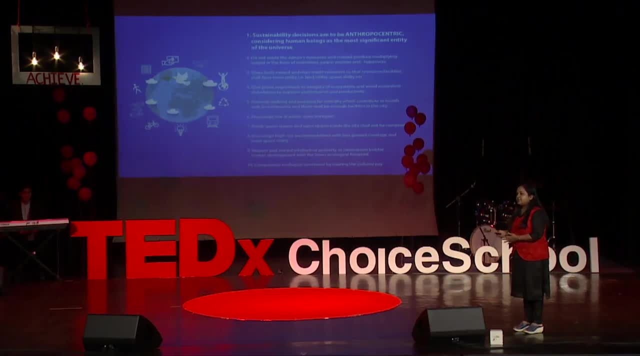 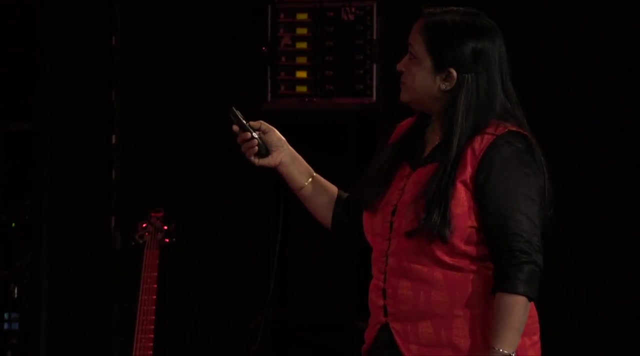 the earth. but in the case of ecocentric, that means human beings will be just like any other animal in this world. that means i believe in all. center for environmental efficiency, or encc. theories are formulated based on the anthropocentric principle: do not waste the nature's resources and instead. 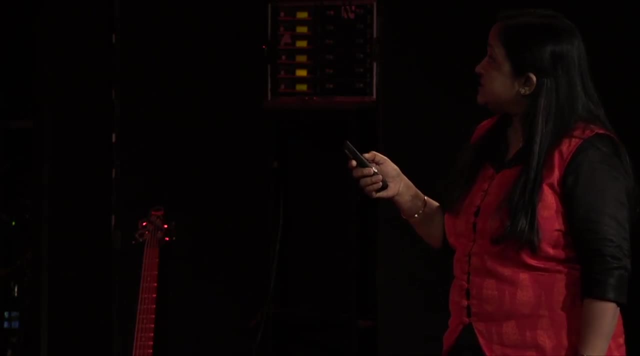 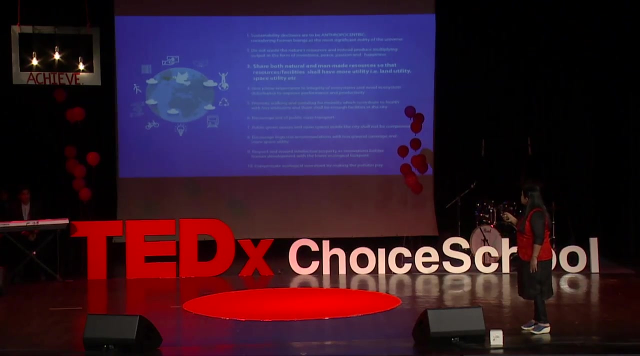 produce multiplying output in the form of inventions, peace, passion and happiness, share both natural and man-made resources, so that resources or facilities shall have more utility: land utility, space utility, etc. because the same piece of land, suppose it is used on different times, the time period, different people. are using land utilities more because more people depends on the number of people who use that. suppose the locked apartments, or locked that is once in, or locked this thing, guest houses. that means it's not land utilities less, it should have more land utility. similarly, face space utility, common apartments, common ownership of land. space utility is more. 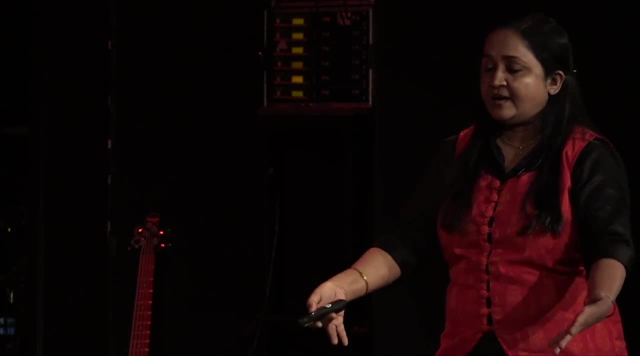 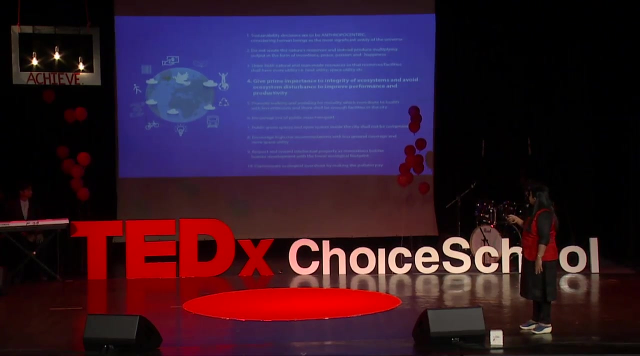 because more number of people are enjoying the facilities given in the system. give prime importance to integrate of ecosystems and avoid ecosystem disturbance, because all these power lines and detergents and what all man made activities are going on, that is in the ecosystems, it all creates ecosystem. 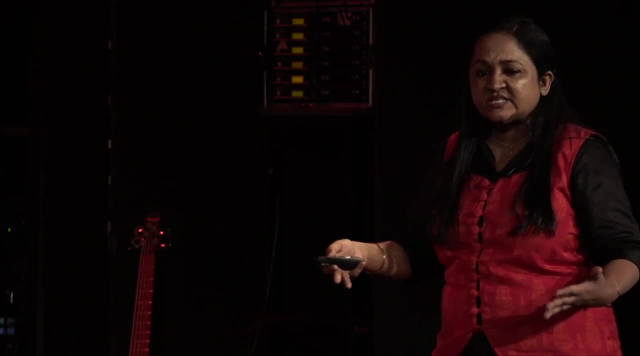 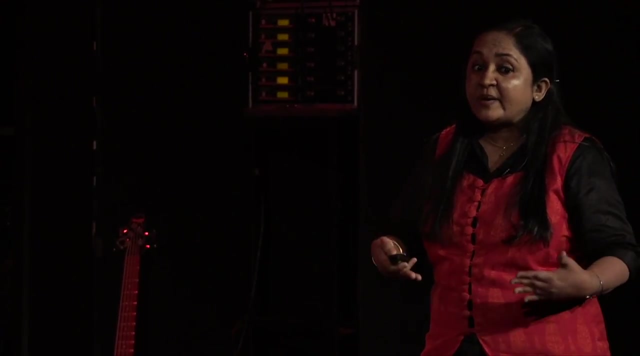 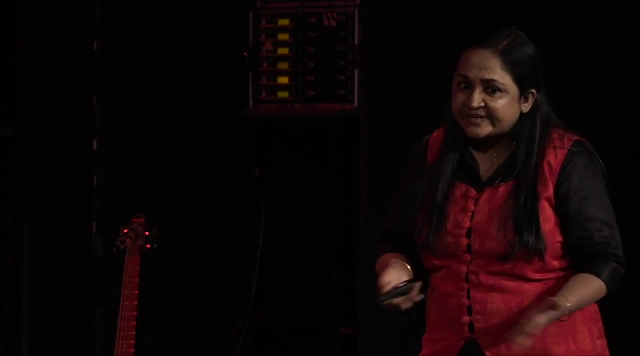 disturbance and it will kill by the microorganisms in the ecosystem, so that ecosystem functioning is not properly, so that there will be productivity loss, the performance loss. that is what is happening in kerala. i must say that because it, because of the scattered development pattern wherever we go, 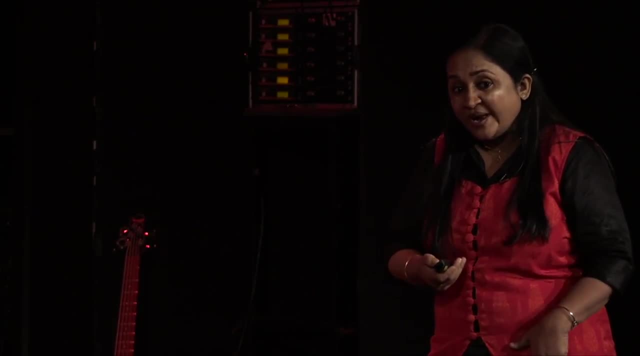 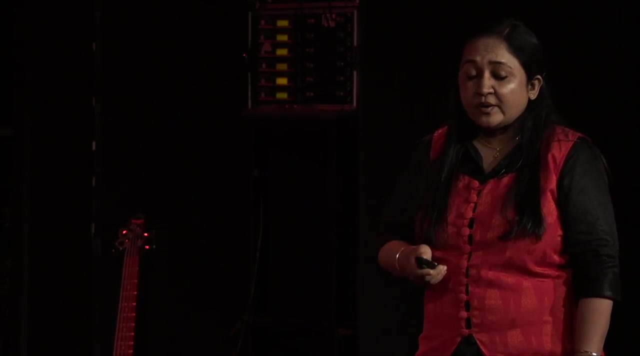 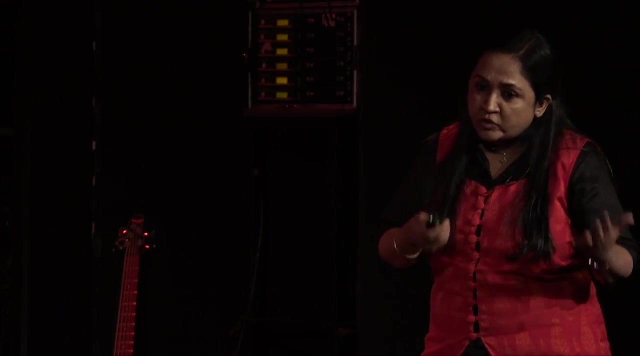 wherever this is, on the mountain top also, we can see the mobile tower, we can see the electrical line and we can see the man-made activities there. so ecosystem, this disturb, ecosystem integrity is the most important thing to have: performance because for our own sake, for man, for his, for his. 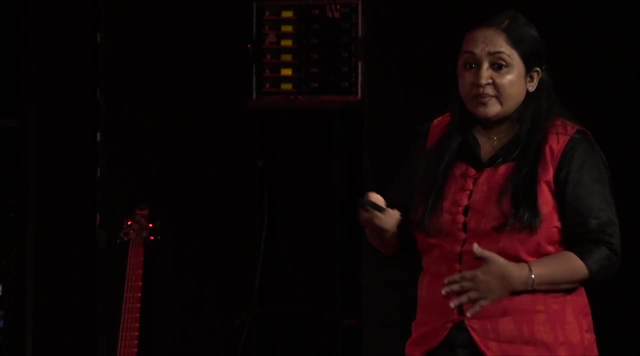 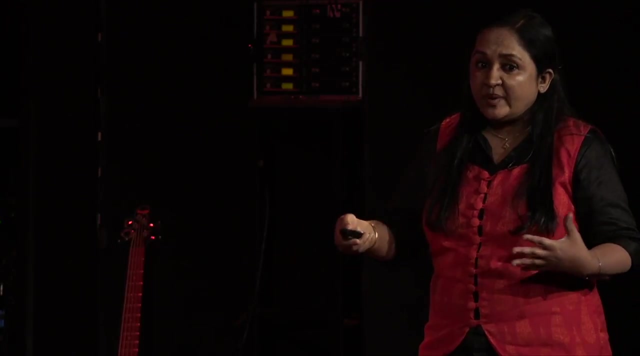 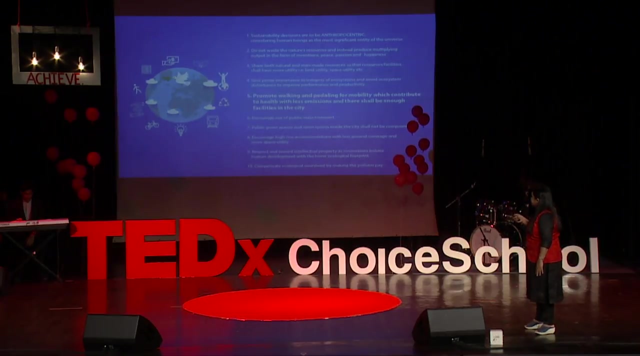 own sake, this kind of ecosystem disturbance should be avoided to so that the in the in the ecosystem will function properly, so that there will be productivity and there will be quality for the ecosystem. promote walking and pedaling for mobility, because walking and pedaling, that is cycling. that is very important. 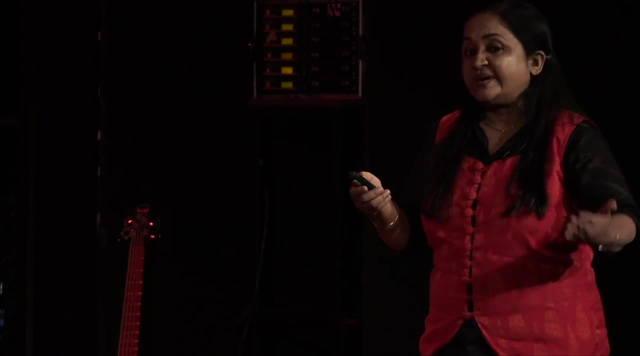 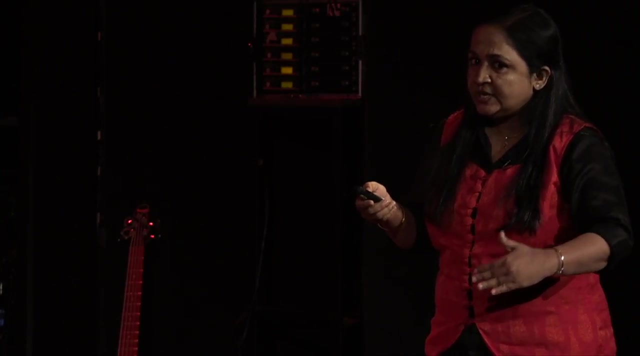 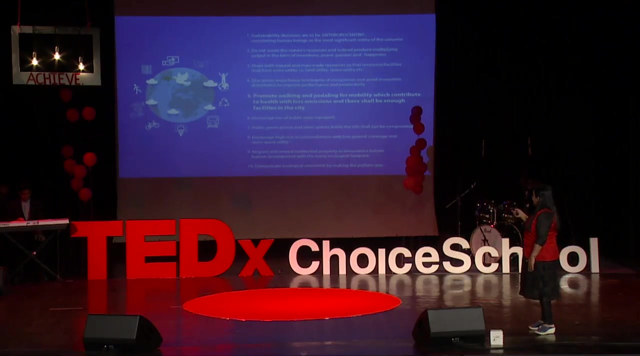 for a city because it contributes to health but it reduces ecological footprint. health is a part of human development, while ecological, that is, energy consumption, is the part of ecological footprint. so both side there will be effect in the case of walking and pedaling and encourage a use, use of public mass transport. again it reduces emissions because more number of people 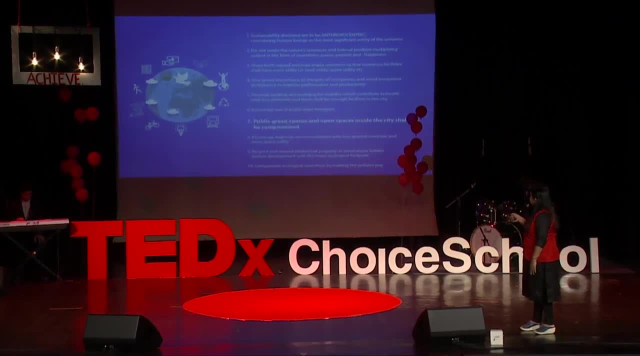 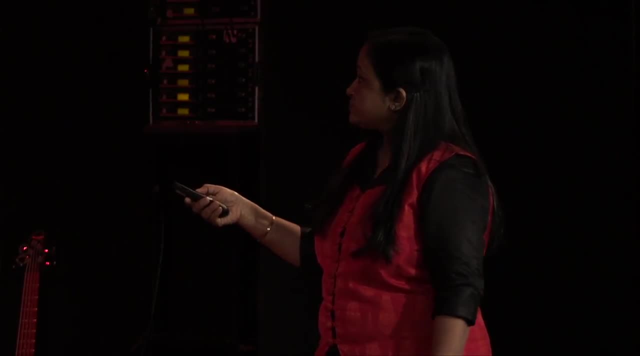 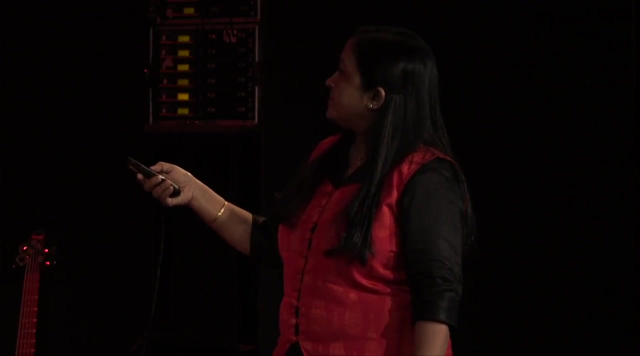 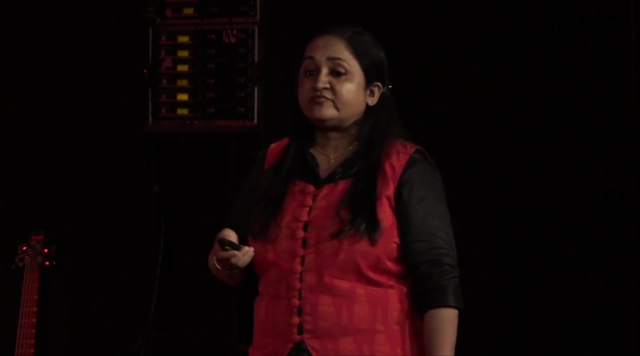 are using. promote green spaces and open spaces inside the city because more number of people will be able to uh the. enable human development. increase high-rise accommodations with less ground coverage and more spatial utility. respect and reward intellectual property as innovations. blaster human development with the lower ecological footprint, because now the population is increasing like anything, and if the 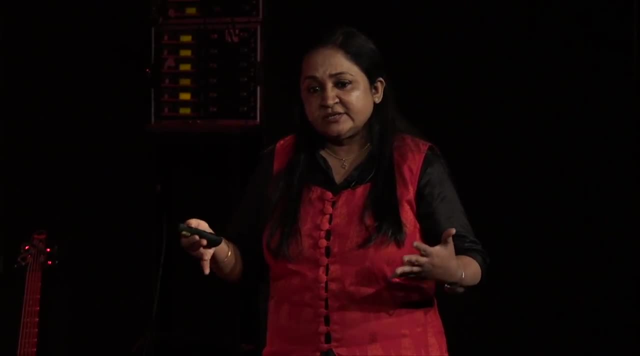 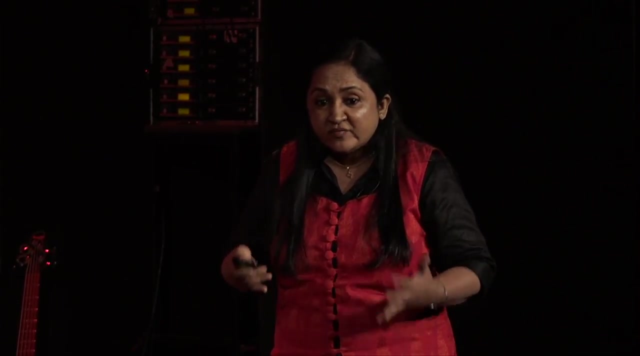 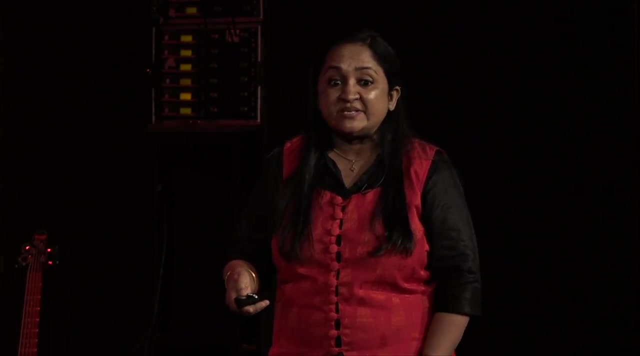 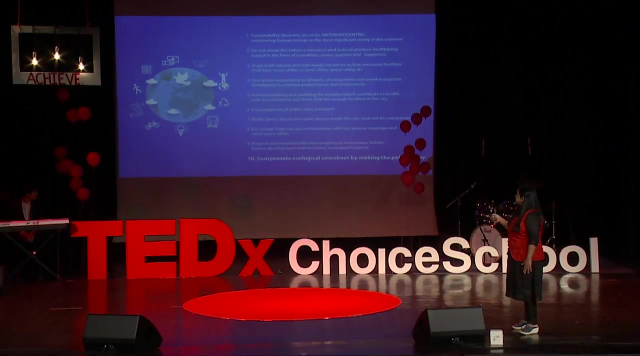 anthropocentric principles are right, then we have to, while protecting all the ecosystems and everything intact. we have to have, that is, innovations: how more number of people can be accommodated in earth without causing damage to the environment. compensate and ecological overshoot by polluted pay. these are the ten commandments, and these ten commandments i have. 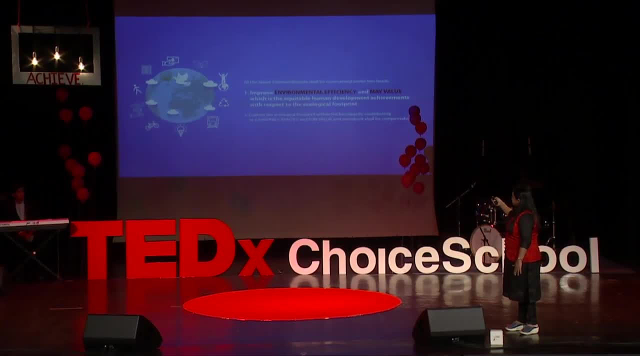 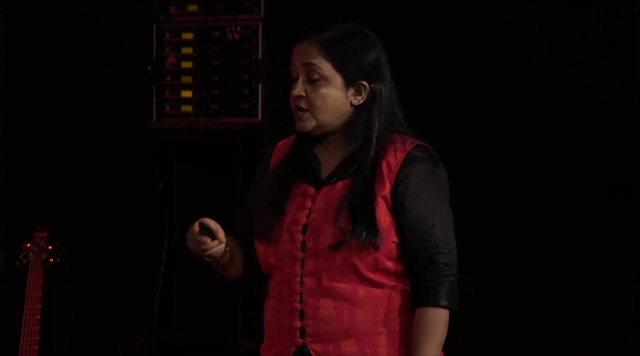 evolved from these two uh, two summarizing commands like: improve the environmental efficiency and may value, and then improve carrying capacity and tone value. and these are the applications level. it has got applications everywhere, from the individual level to global level, from the world, country, state, region, city. all these actions are to be done from the government, in the case in the, in the in the form. 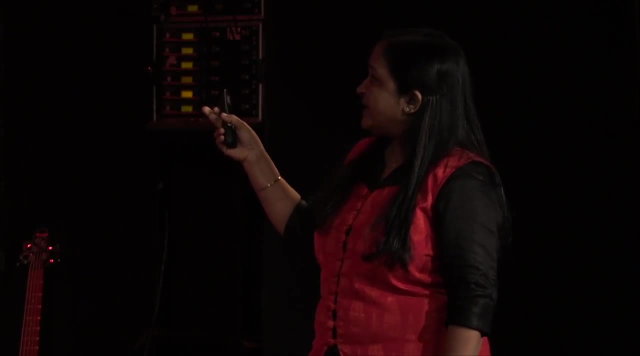 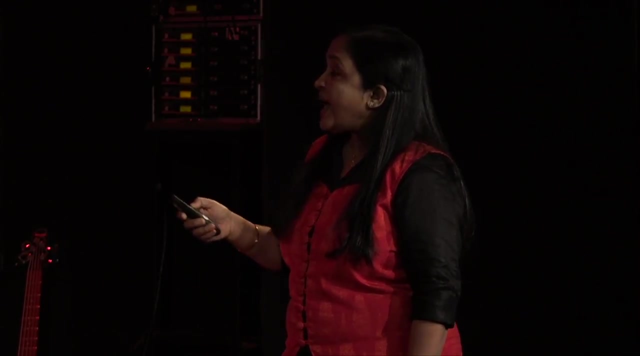 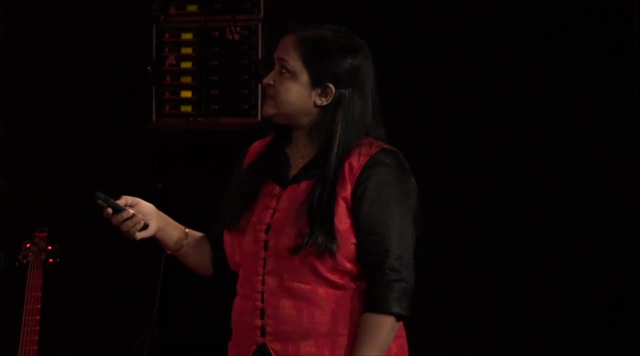 of policies and projects, while at the bottom level, action from bottom, it should be ヒブレイト- action from people, or how it should be at the individual, family and community level. what, what we can do? what are all the tips? small tips: reduce the energy bill, that is, use of solar. 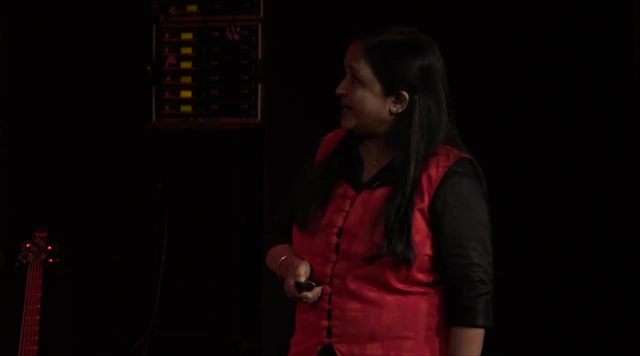 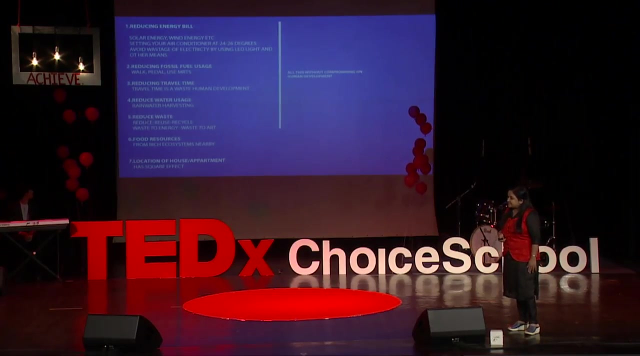 energy and wind energy. that is a non-renewable energy. renewable energy and setting up of air, air booming. the Aug 14 acko Enjoyment B κ of teka b buta bond. do not put the AC below 25 degree, because 25 degree is more than enough. why 16 degree? 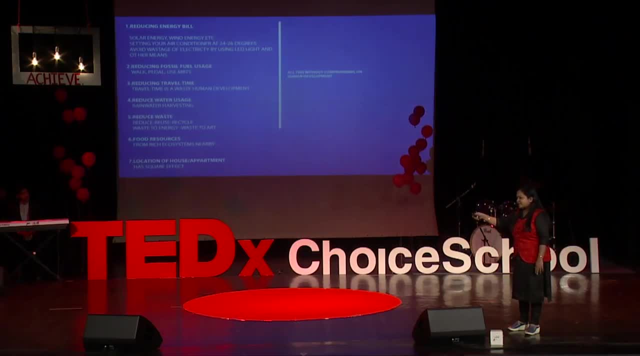 and putting a set is and it is going to the all. the heat is going to the outside, and outside people also will be prompted to use AC. then what will happen at the end of the day or end of the year? because that should be our policy, then avoid wastage electricity. 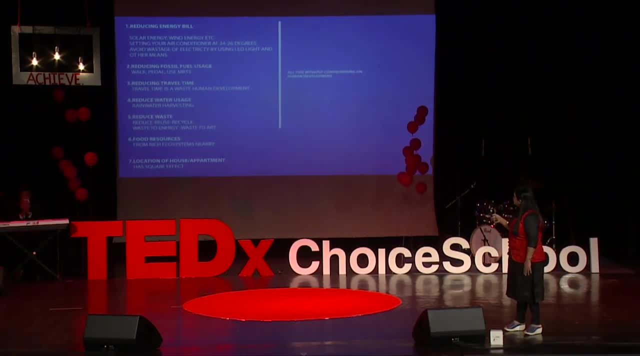 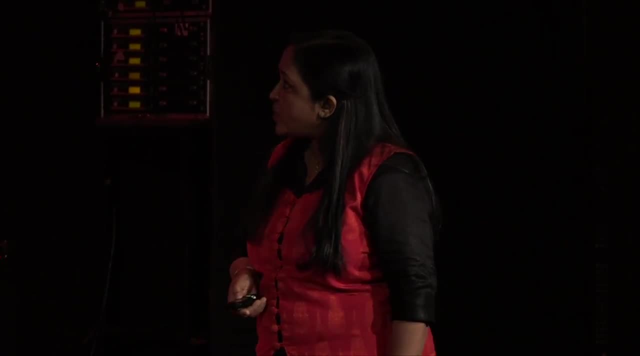 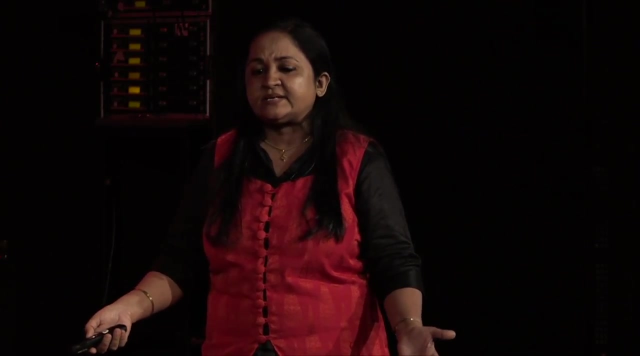 wastage of electricity will using LED lights and other means. reducing fossil fuel usage by walking, pedaling and use of mass transport. reducing travel time. travel time is a waste of human development because we are simply idling in the, that is, vehicles, so reduce 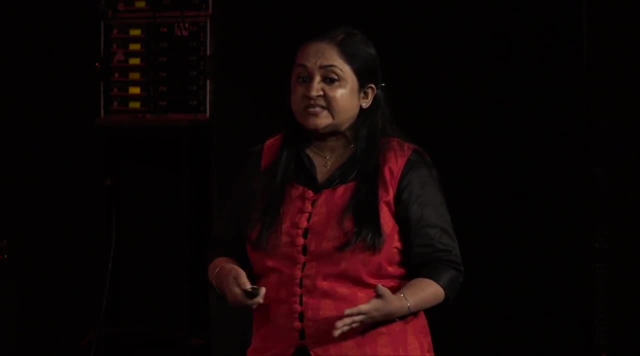 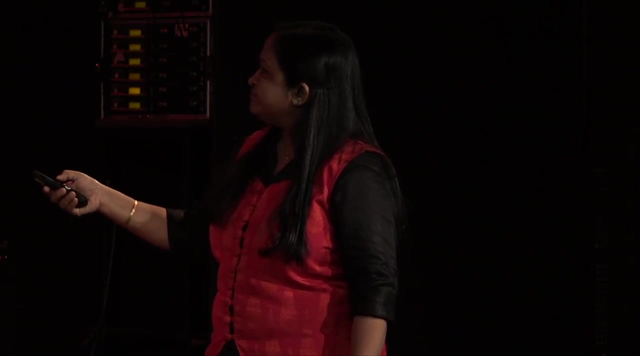 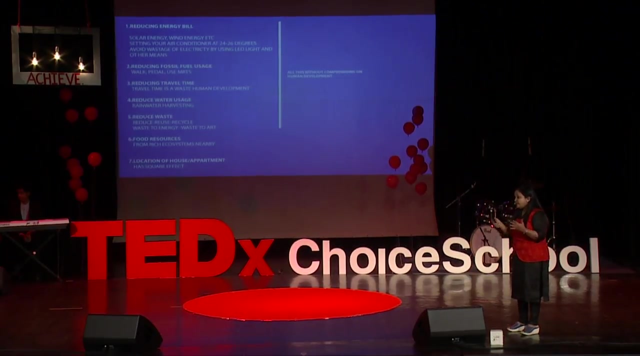 the travel time. so our house location should be in such a way that our travel time should be reduced for all the families. then reduce Reducing water usage. that is, rain water harvesting can be done. rain water harvesting- that too can be done. first, water shall be collected on the rooftop so that pumping 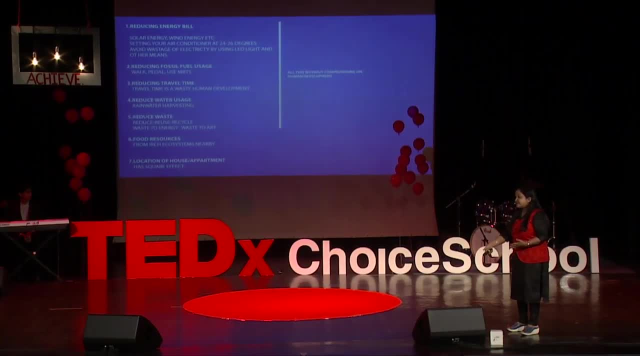 can be avoided, then the balance: water can be collected at the sump and again the balance can be, that is, underground recharge. Then food resources. we should take food resources from the nearby rich ecosystems because the transport, Transport, Transport. 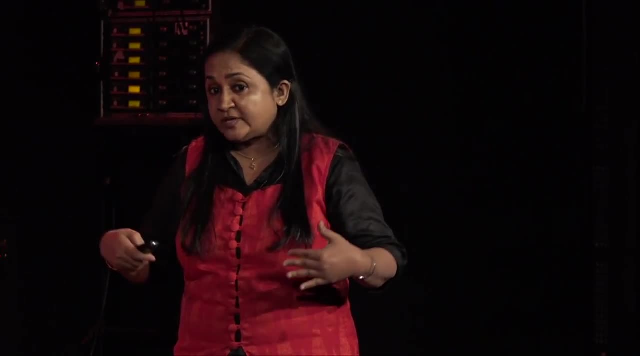 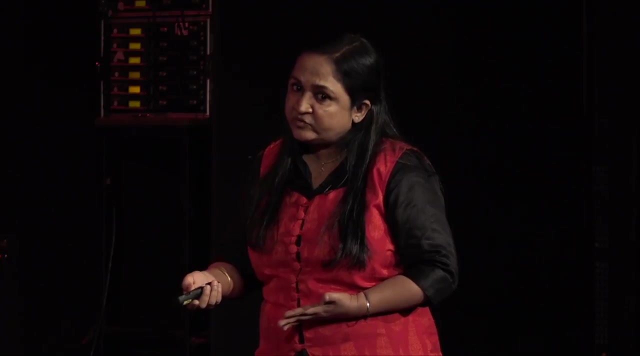 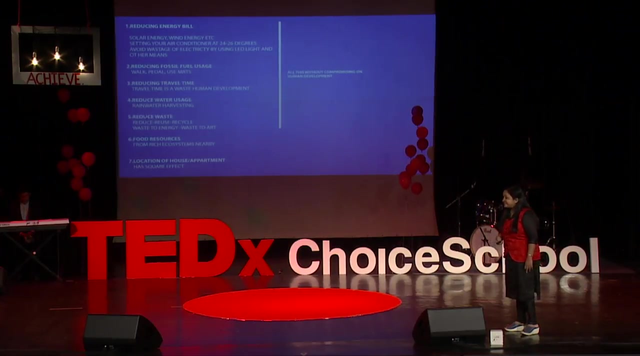 The food which is transported from that is far away places. it reduces the food value, which affects the health. at the same time, it increases the ecological footprint because of the transportation, then location of the house or apartment. it has got a square effect. 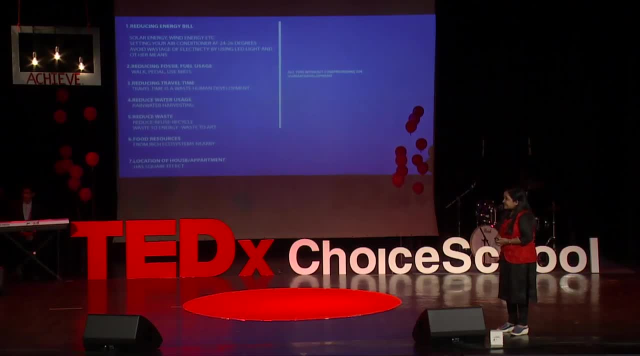 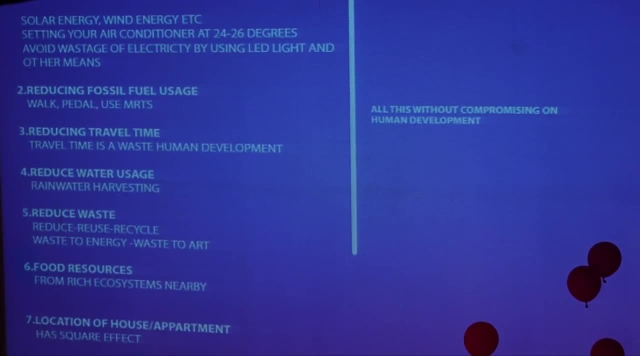 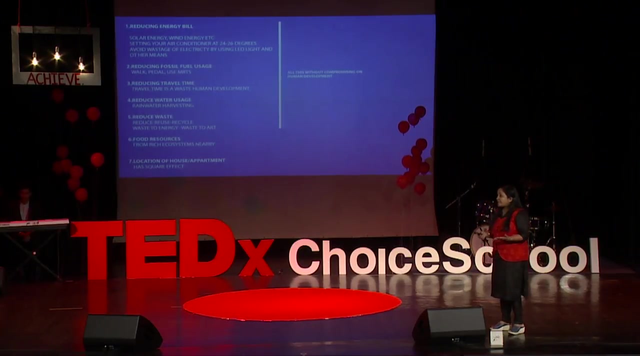 square effect means it is, that is, it increases, because if our house is located in a very environmentally efficient location and with all such schools, colleges and all such hospitals and railway stations and things like that, if it is nearby, it is known as. 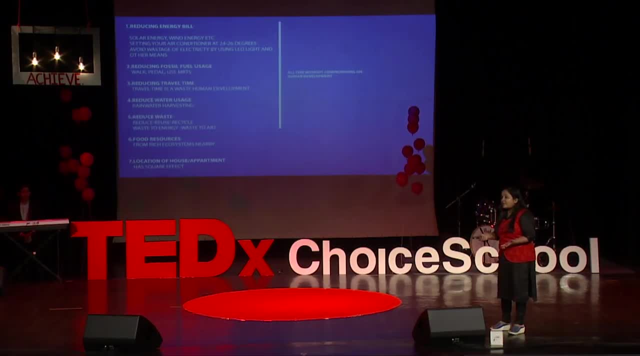 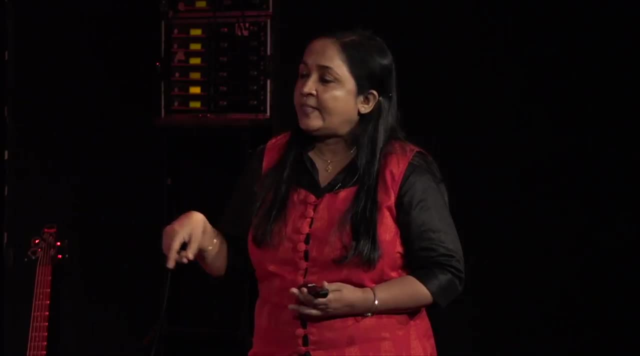 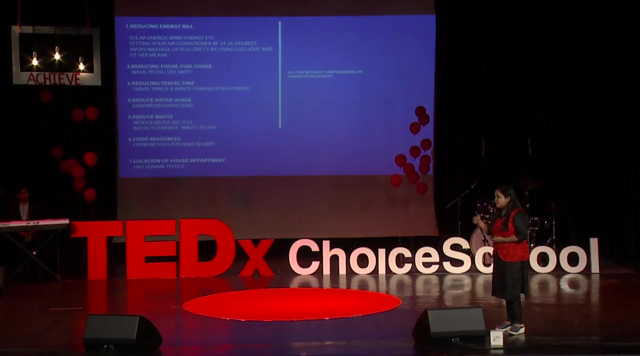 an environmentally efficient location. that means our human development opportunities will be high while ecological footprint is reduced. that means square effect is there. It is known as alpha square effect because accessibility is a very important factor. I have named in my thesis it as alpha, so alpha square effect because that multiplying 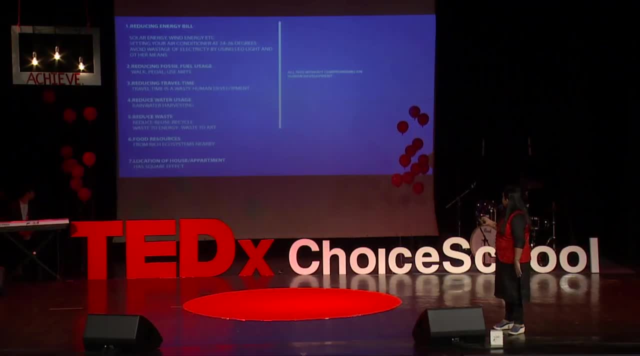 effect is there for the location of the house. And all these reducing, reducing, reducing things. these are all without compromising human development, because if we need it, we use it, avoid wastage, and so that all emissions will be brought back. either it will be the input will be reduced, or it. 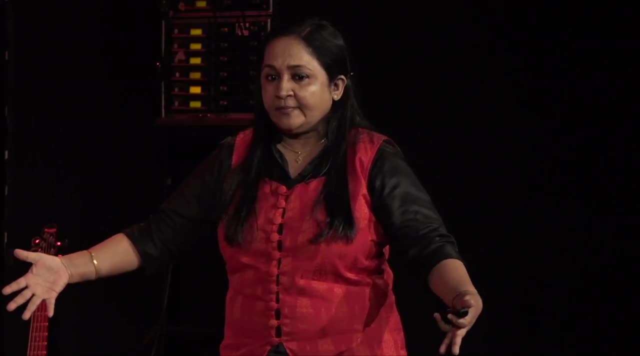 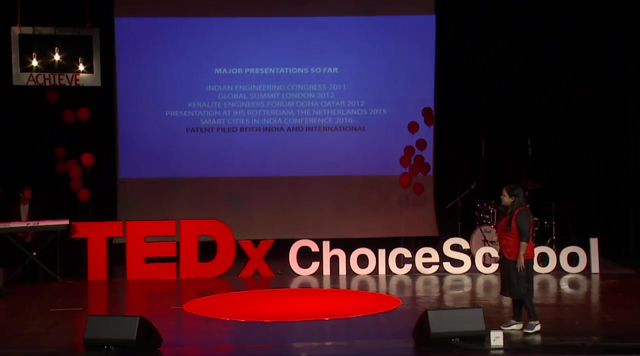 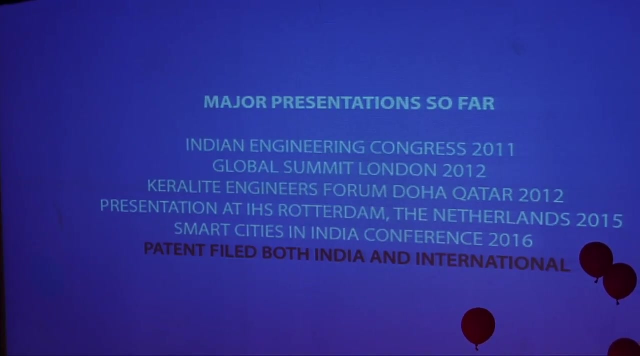 can it brought to the output so that it will be functioning, it functioning with the environmental, high environmental efficiency. And I have made presentation. This is the presentation which I made, action from people and so far I was making presentation in different places with the action from the government and I have made presentation for. 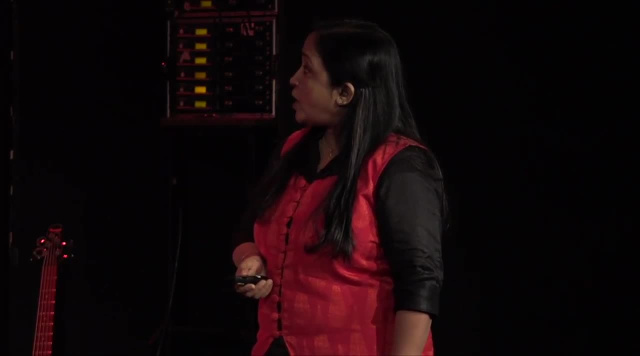 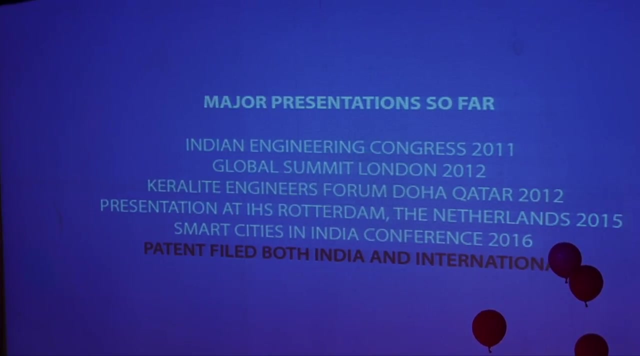 at Indian Engineering Congress 2011,. Global Summit- London 2012,. Keralite Engineers Forum- Doha, Qatar, 2012,. presentation at IHS Rotterdam, Netherlands in 2015,. and Smart Cities in India Conference 2016 at New Delhi. 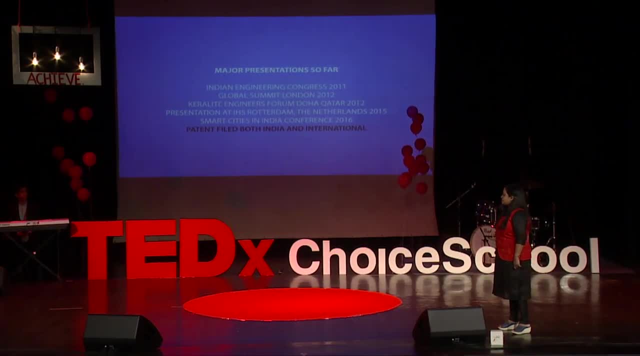 Thank you. And patent also. I filed both India and international and Indian patent. it is published and international patent patent pending number I am waiting for And my achievements are, that is. these are only one part. I have explained. 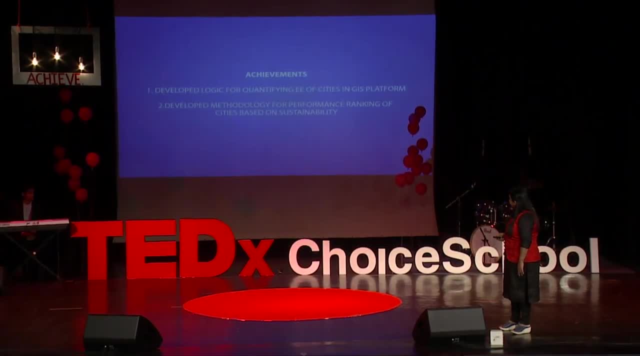 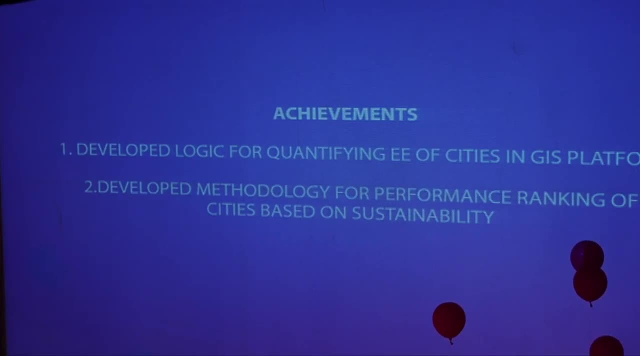 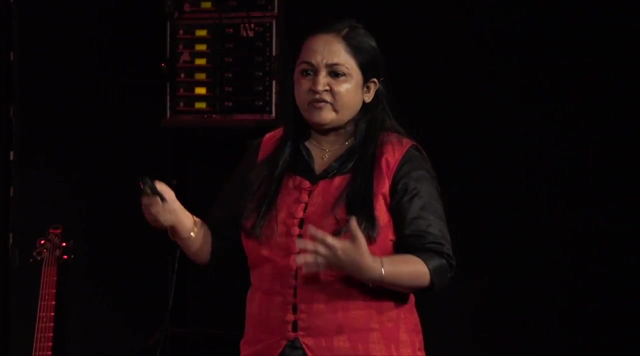 My achievements are: developed a logic for quantifying the environmental efficiency of cities in a GIS platform and developed a methodology for performance ranking of cities based on sustainability, Because in India, if there are so many cities based on environmental efficiency and carrying capacities, we can quantify it.